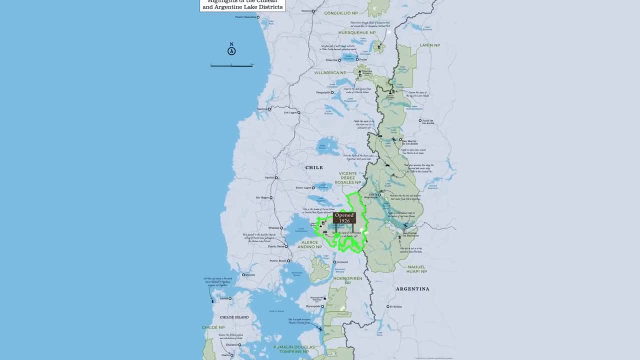 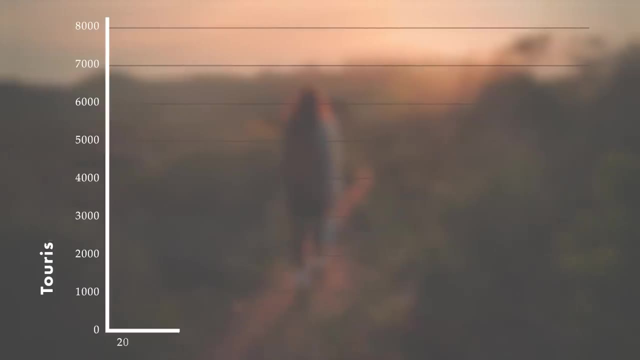 followed by nine more parks. during the last century. As one of the most attractive hiking regions in South America, the Lake District played a big role in Chile's tourism industry, which had its peak in 2017, with nearly 7 million international travelers arriving. 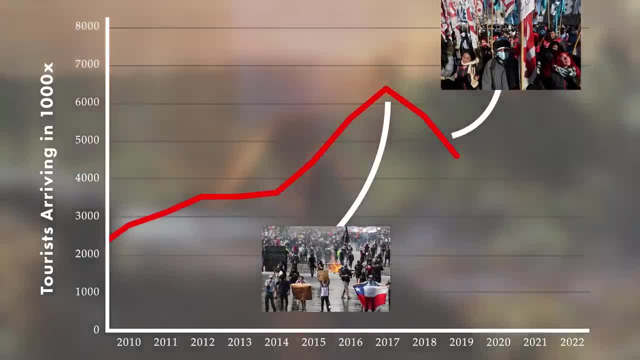 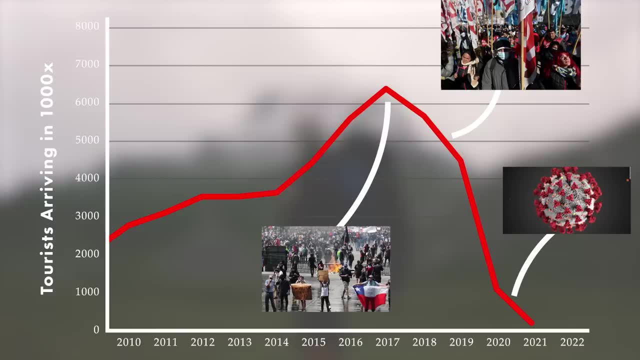 A series of internal unrests: the Argentinian monetary crisis, which prevented the largest group of tourists from traveling, and the COVID-19 pandemic have reduced this number to a mere 190,000 tourists in 2021, throwing the region into a deep crisis. The Ministry of Tourism, however, 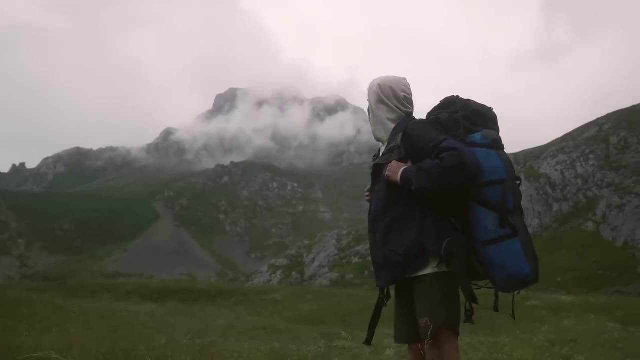 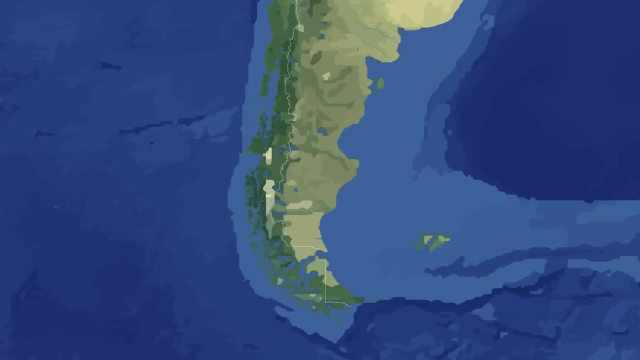 hopes that the numbers recover to pre-COVID numbers by 2024, giving the livelihood back to the 600,000 Chileans which are dependent on tourism Next to lakes in the Lake District- the area's stratovolcanoes. the Lake District and the Lake District- the area's stratovolcanoes. scattered over the plains are another reason for why tourists flock in in the millions. Villarica, Osono and Lanin are just some of the year-round snow-covered cones which even offer little skiing resorts and challenging ski-touring routes in the winter. 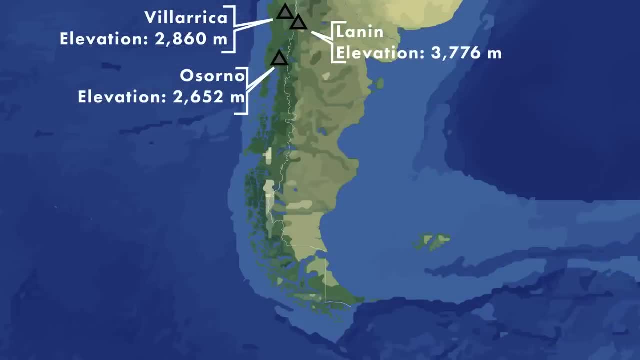 Lanin is the highest mountain, for hundreds of kilometers, and as such it marks the border between Chile and Argentina. This principle has been applied to almost all the highest peaks of the Andean Mountains, which neatly split the mountain range between the two countries. 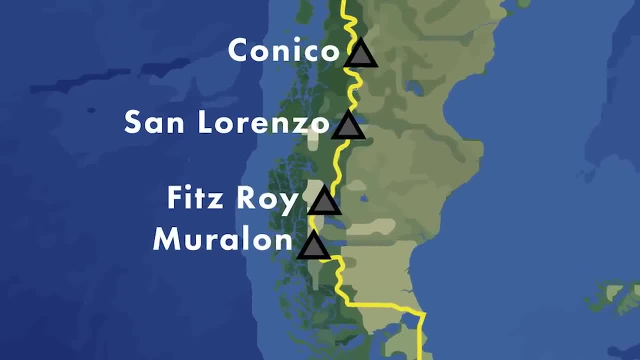 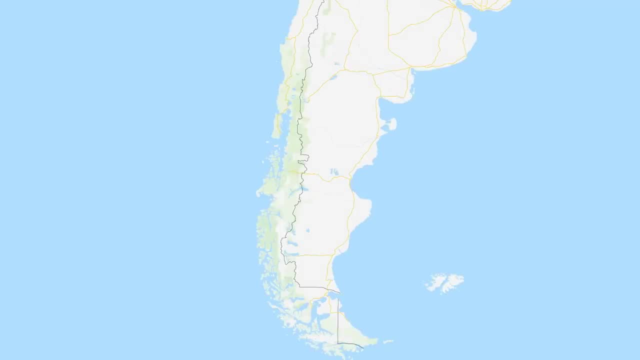 Following the Patagonian peak southwards, we enter the third region of Patagonia, Chapter 3, the ice fields. During the last global cold period, most of the Lake District and every mountain and volcano from today's Santiago de Chile down to Tierra del Fuego has been buried. 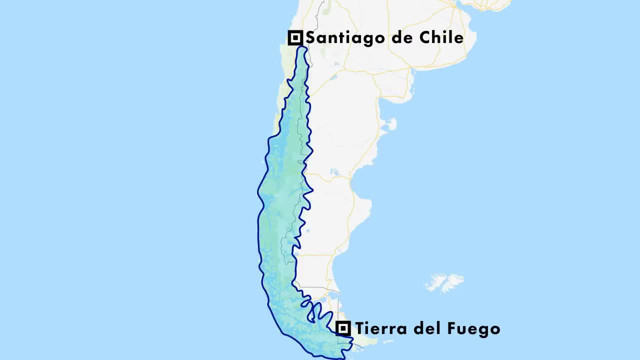 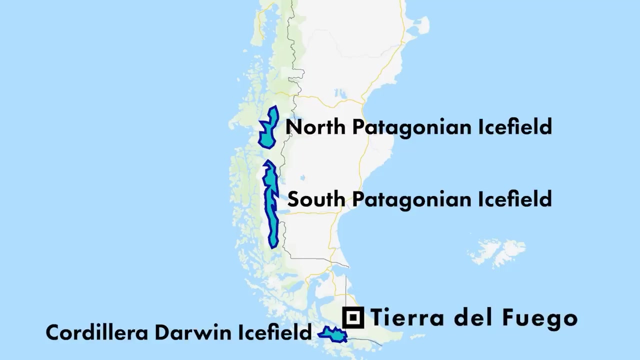 by a thick slab of ice. The Patagonian ice sheet used to have a volume of 525 cubic kilometers, but this has been steadily declining since its last maximum, 21,000 years ago. Today, only three can be found between the summits of the southern Andes, and it is estimated that the retreat of 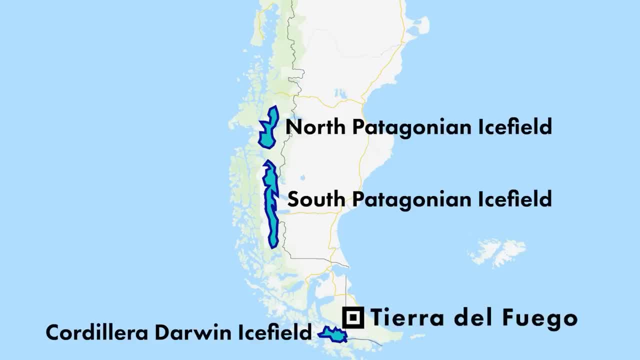 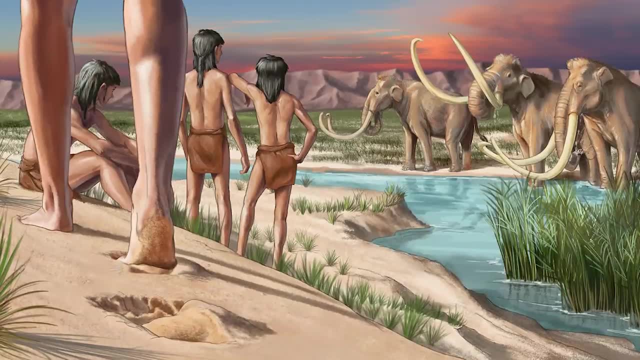 the Patagonian ice masses alone has contributed to a sea-level rise of 1.2 meters during this time. While most of this shrinking occurred when humans were still in their caveman days, humanity's influence here is undeniable. Researchers have meticulously documented. 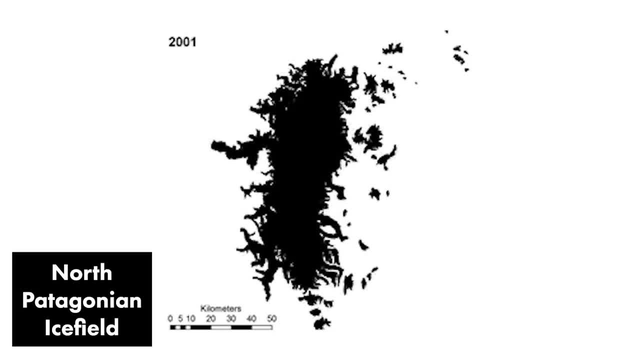 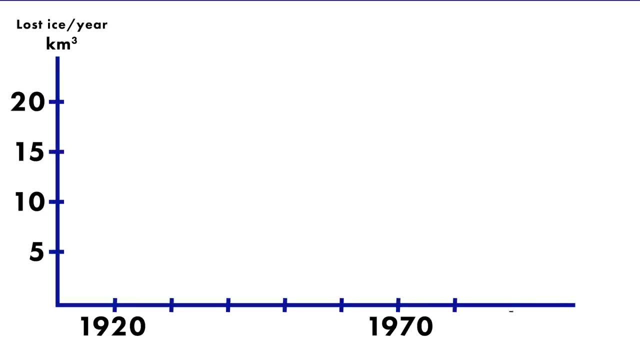 the retreat of these ice fields for the past 100 years, providing us with tangible data on the impacts of global warming in real time. The combined ice masses of Patagonia lost around 6 cubic kilometers of ice per year around the year 1900, but this number has 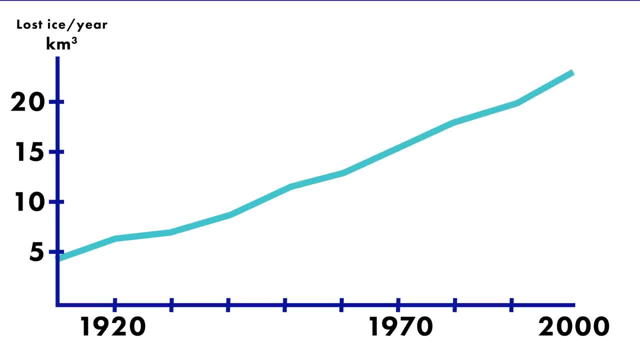 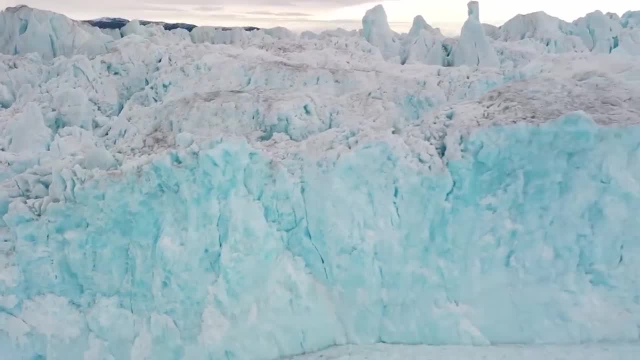 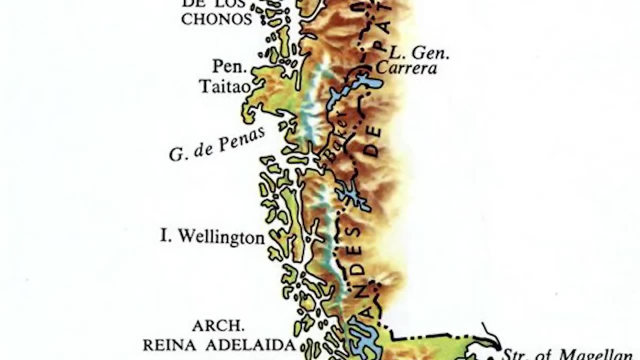 skyrocketed to around 15 by the 70s and 24 by the turn of the millennia. If, or more accurately, when, these ice masses will be completely gone is up in the air for now, but the trends do not look promising. The core of the Patagonian ice fields lay at elevations of over a kilometer in the 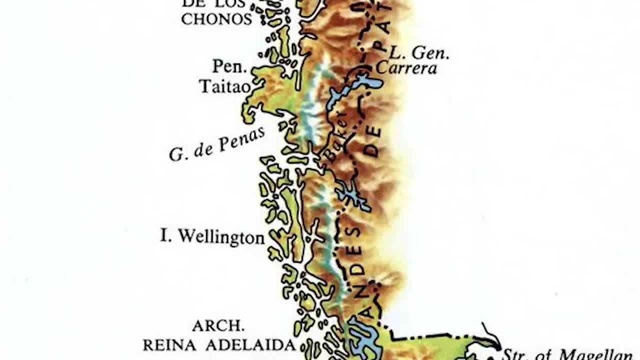 center of the Andean mountain range, but due to the retrieval of the ice, the distance to the fjords are just a few kilometers. in many instances, The resulting steep slope actually creates some of the fastest flowing glaciers in the world, with the fastest arms, traveling at speeds of 28 meters per. 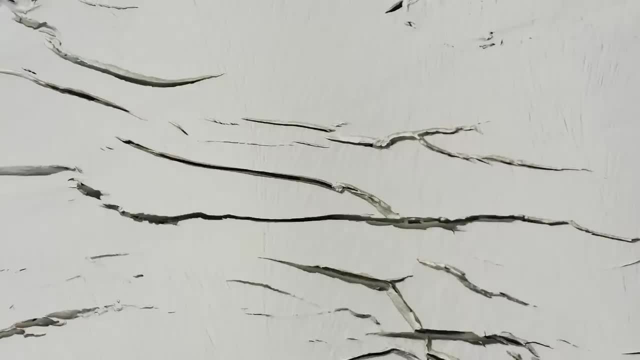 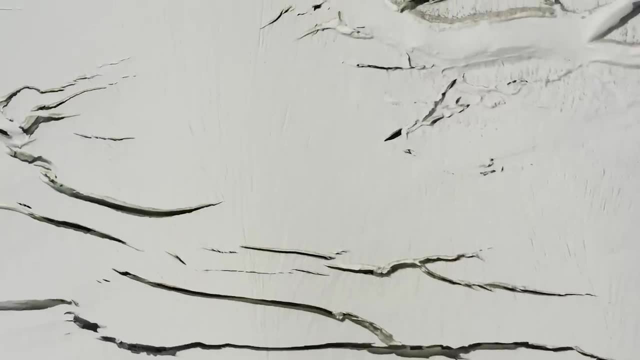 day towards the ocean. While it is sad that the Patagonian ice is one of the fastest disappearing glaciers in the world, its recess reveals another incredible part of Patagonia which now has become accessible, bringing us to chapter 4, the southern fjords. Similar to the dramatic landscapes found, 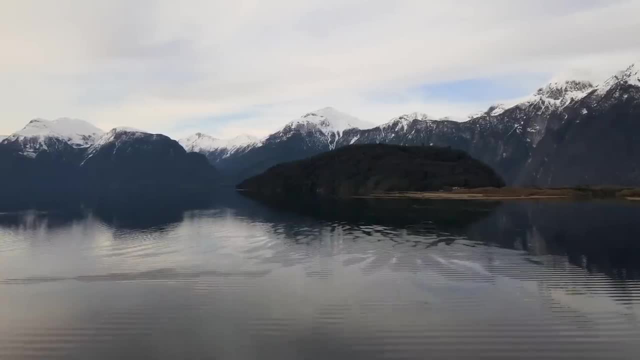 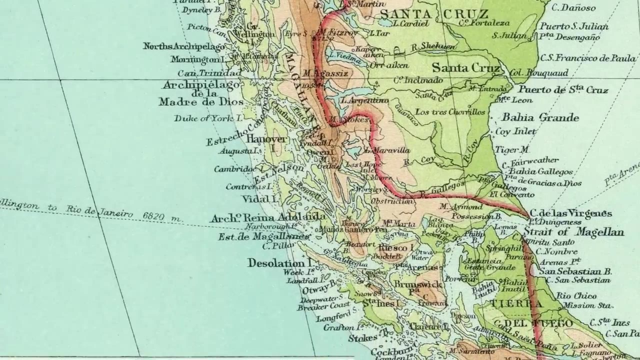 on the island. Patagonia's fjords are a testament to the powerful sculpturing forces of glaciers over thousands of years. Valleys carved by ice and flanked by steep cliffs and mountains have created a complex network of waterways, and the surrounding ecosystem offer a rich field of study. 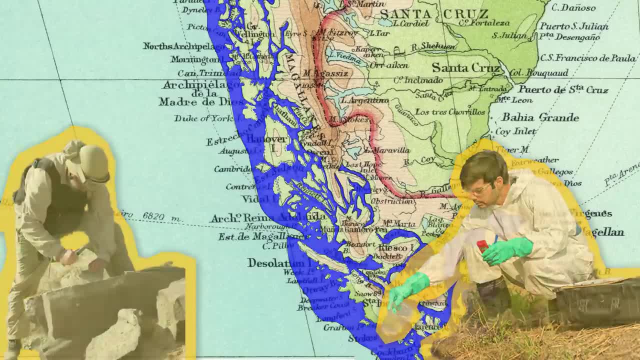 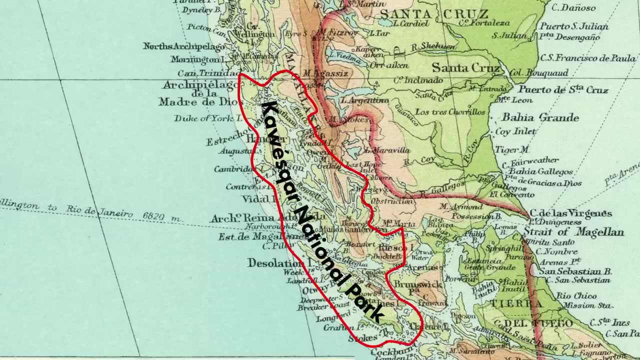 for environmental scientists and geologists alike, To protect the pristine landscape. most of the fjords have recently been put under protection in the form of the Kaviskuan National Park. Encompassing over seven million acres of fjords and islands, the Kaviskuan National Park is 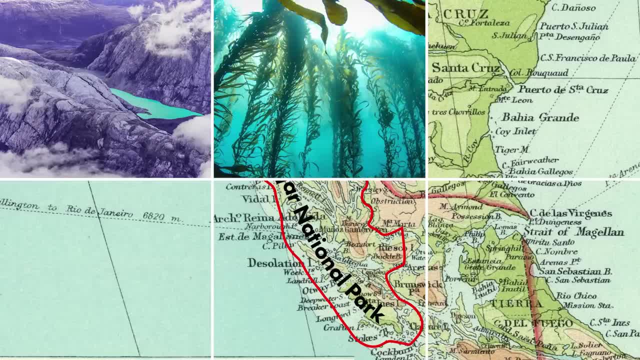 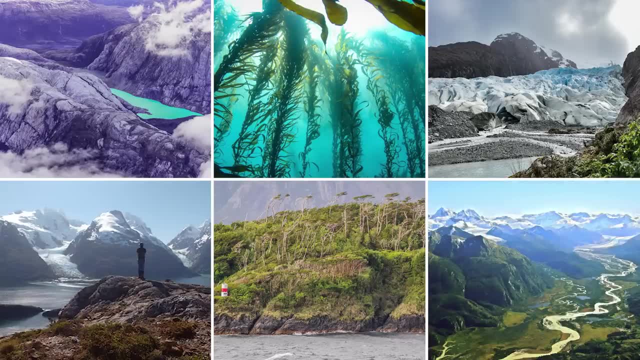 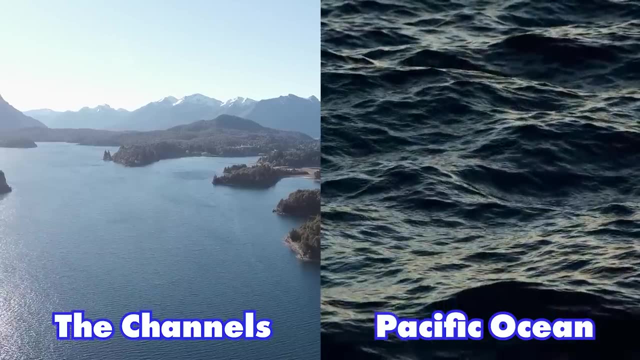 a mosaic of massives underwater kelp forests, glaciers, fjords, wetlands and valleys, Basically a more concentrated version of Patagonia. within Patagonia, The channels are used by many smaller vessels to avoid navigating the sometimes rough Pacific Ocean, and the fjords have been navigated. 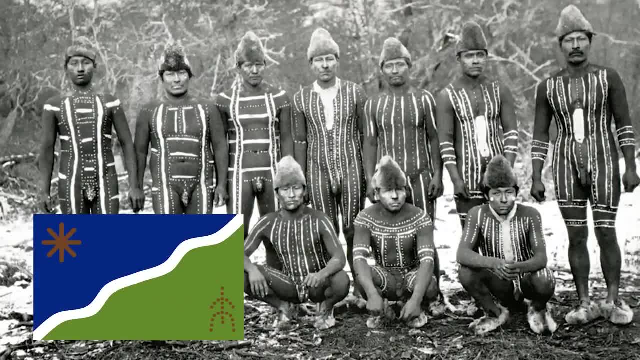 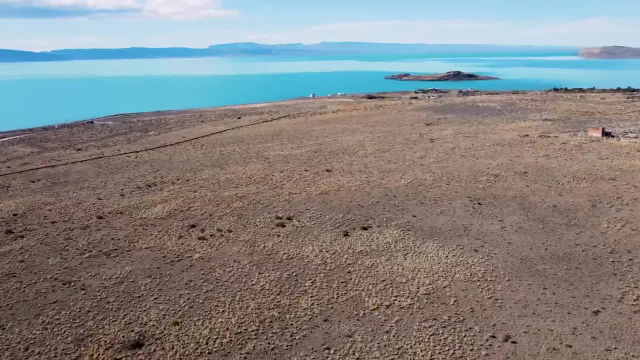 for over 7,000 years by the Kaviskuan people, in whose honor the park has been named. Millions of years of glacial erosion has created the hundreds of islands, but despite its remoteness and harsh environment, many fascinating mammals actually call these almost untouched lands their. 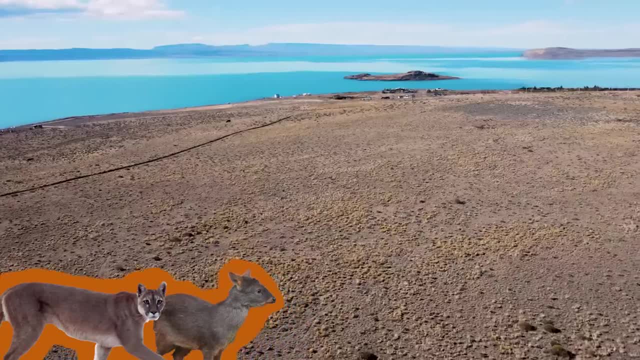 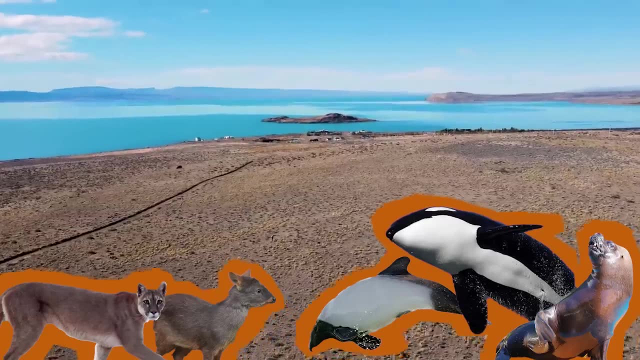 home From pumas and tiny deers called pudu on land, to dolphins, sea lions and orcas in the adjoining Marine National Reserve. the Patagonian fjords are one of the last true wildernesses on the planet. Having explored the Patagonian desert, the beautiful lake districts of Chile, 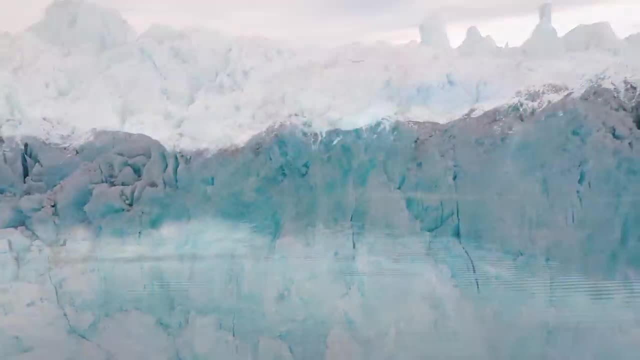 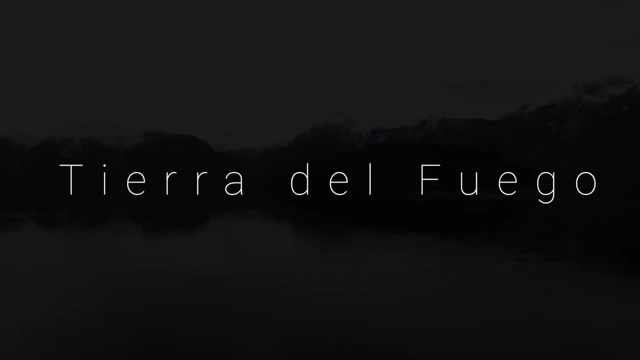 and Argentina, the fragile ice fields and the majestic fjords. one last region is missing to have the complete overview of Patagonia, and that is Chapter 5. Tierra del Fuego. With latitudes reaching 56 degrees south, Tierra del Fuego encompasses the southernmost 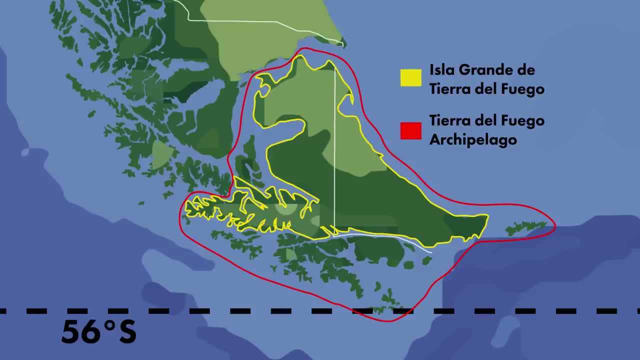 landmass outside of the Antarctic continent. As such, you can find the southernmost city, Ushuaia, the southernmost post office in the Tierra del Fuego National Park and the southernmost airport at Puerto Williams, When translating the remote archipelago's name, Tierra del. 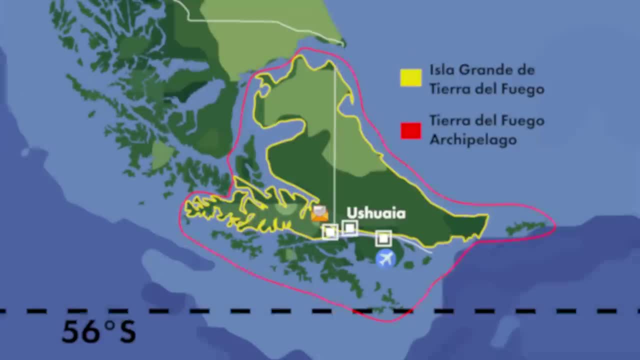 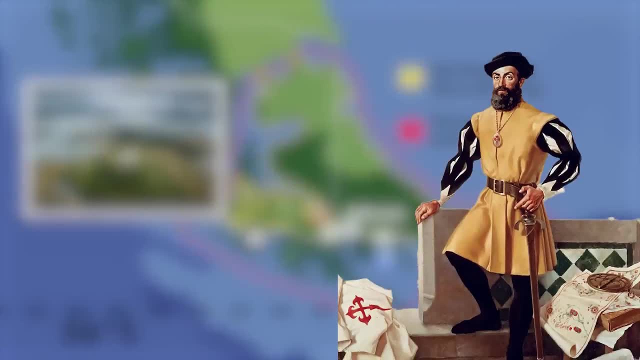 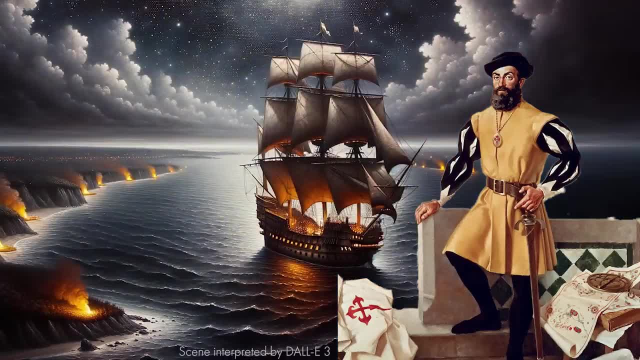 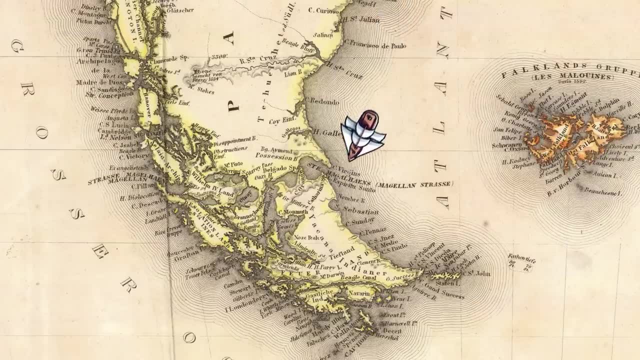 a series of bonfires on the shores lit by the indigenous population of the islands. For the coming centuries, the region has been left alone by Europeans and only functioned as a practical waterway connecting the east and western shores of the Americas. since the 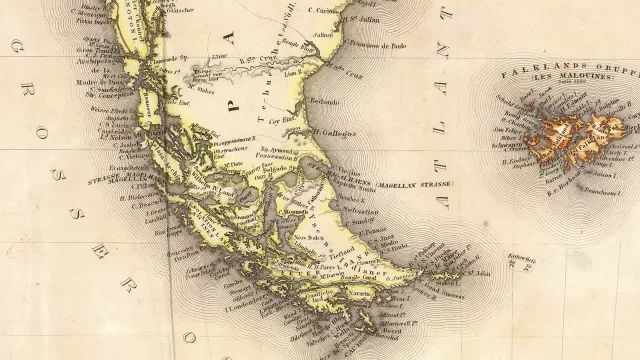 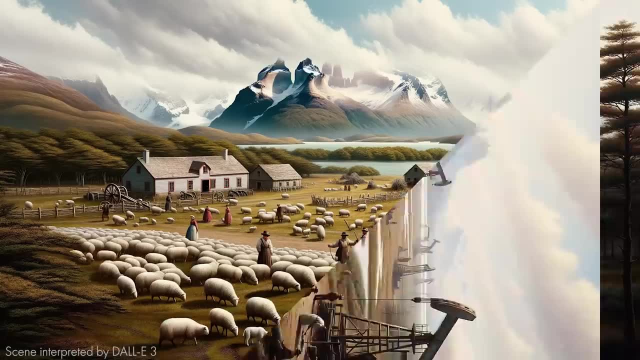 Panama Canal only opened inычно. Repeat this translation, but fell嘻 14.. Tierra del Fuego gained recognition during the Patagonian sheep farming boom in the late 19th century, and today the economic focus has shifted to petroleum extraction and tourism. 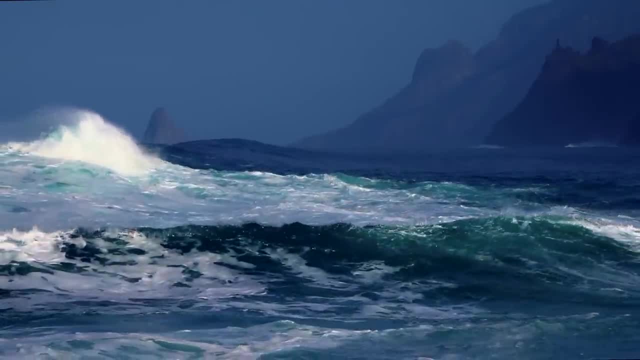 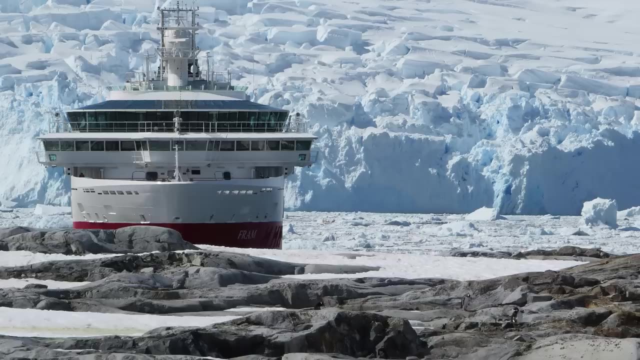 These tourists do not typically come for the weather, which boasts year-round temperatures around the freezing point, constant heavy winds and extremely high precipitation, but instead it's used as a gateway to the Antarctic. For Muxihuaya, it's only 1100 km to the outer tip of the Antarctic Peninsula, and many scientific 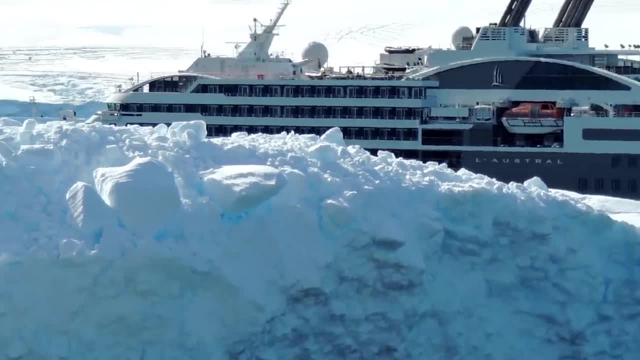 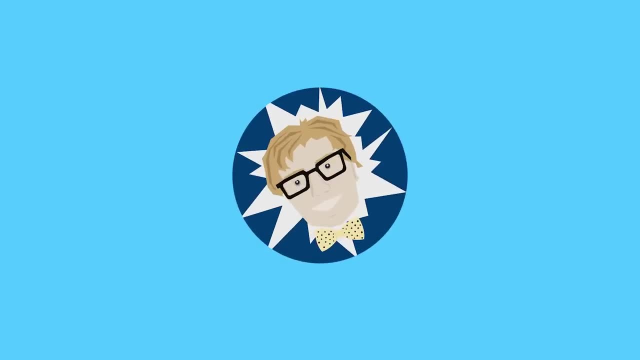 explorations, and cruise ships are making use of this favourable location. If you want to continue learning about the Antarctic continent, you should check out this complete guide to the Geography, History, Politics and Science of Antarctica, or check out the video which the YouTube algorithm thinks is best for you. 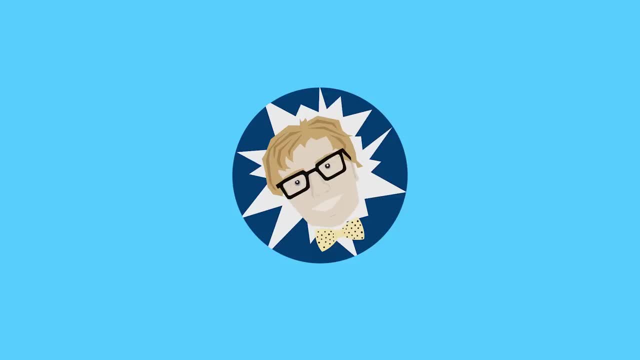 I hope you enjoyed the video and if you want to see more like it, be sure to subscribe and leave a like. Cheers.